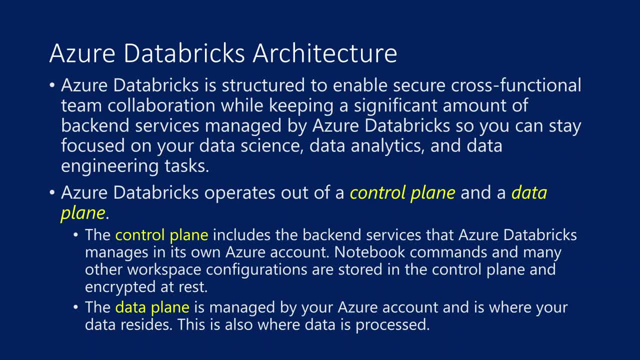 From there, Power BI reporting will happen. This is the general flow. So all this we have discussed already. So, if you think practically from all our past videos, we simply created Azure service- That means Azure account- And then we simply created something called workspace. 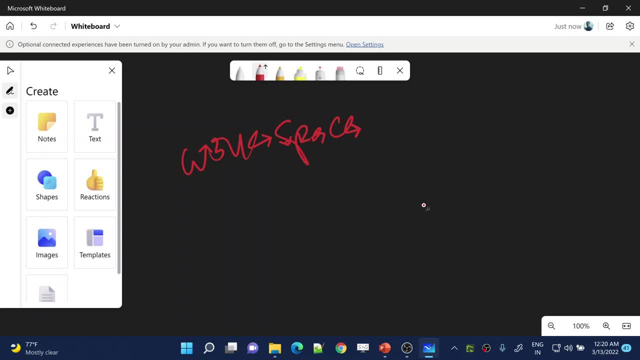 And then, in the workspace, we directly started writing our notebooks. Okay, So this is what we did, Uh, but we have, and also we, we, we kind of spinned up the clusters also, right, So, using clusters only, we created that everything. 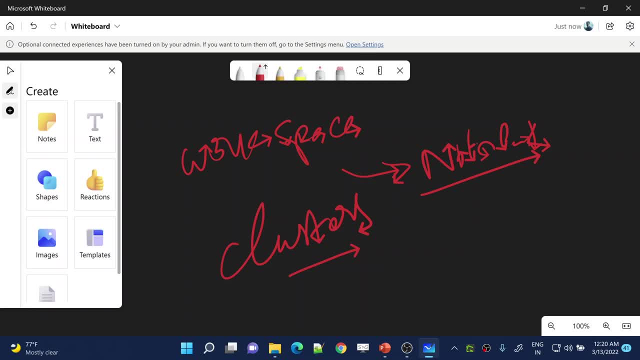 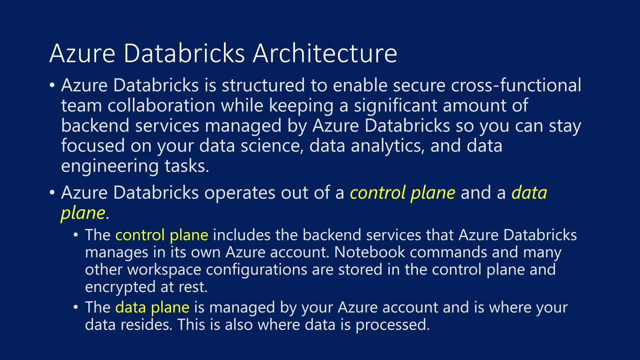 Uh, and the notebooks will be connected with The clusters and to to execute that logic. But if you think, practically we haven't done anything, I mean there is no nothing backend installation or something we did. Everything was handled by cloud. 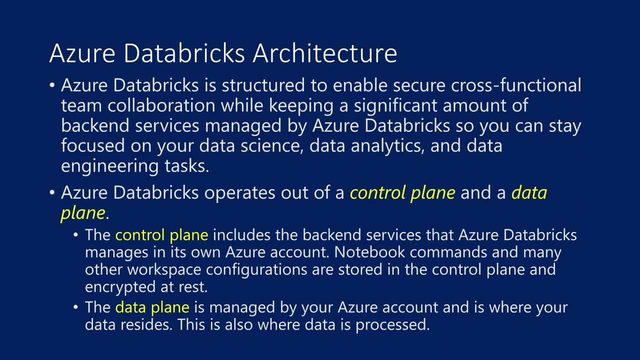 So that is what, uh, it means. So in the Azure Databricks, what will happen? right, Most of the backend services that need your data processing to work will be handled by Azure Databricks itself. You only create the database account and directly focus on writing your notebooks to perform that big data processing. 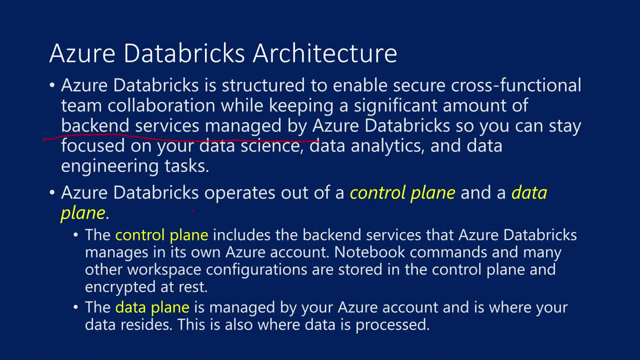 That's it, Okay. So, because of this reason, actually, Azure Databricks operates on two things: There is something called control plane and there is something called data plan. So these are all the two areas which will contain in the architecture of the Azure Databricks. 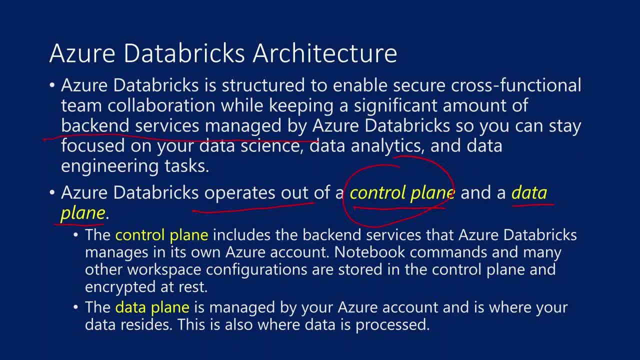 So control plane is the one where Databricks will handle all the backend services. Uh, you can think like control pane is something like Azure Databricks own account. So Azure Databricks will have its own Azure account. In that own account it will have all the backend services that will make your Databricks to run properly. 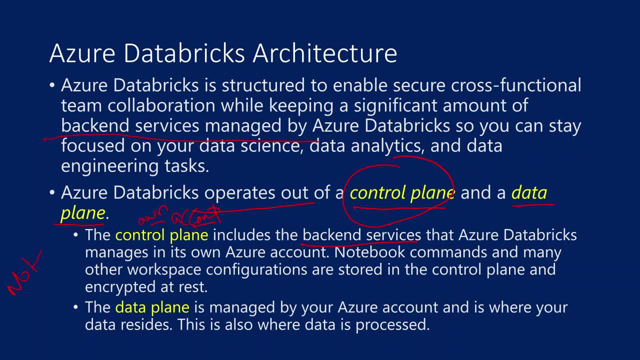 So in that control pane it will contain all your notebooks, metadata and also whatever the workspace configurations you did and how you should do your notebooks using jobs, and all Every information, all the workspace configurations and everything will be in the control pane. 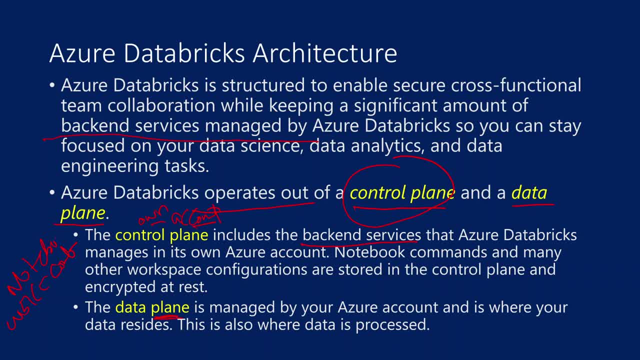 In the data plane. you will have simply uh your data, what you process, All your data will be actually resided In the data plane already and this data plane will be inside your own Azure account. So you can think like control plane will be inside the Databricks account, inside the Databricks account, uh Azure account and data plane will be inside your own Azure account. 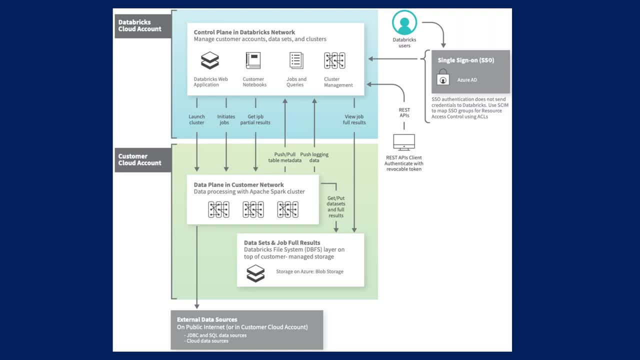 So the same thing I have explained here. Also, if you see this architectural diagram, you can see this is this entire box. whatever you are seeing, this is like a control pane. So, and you see, this control pane is in the Azure Databricks. 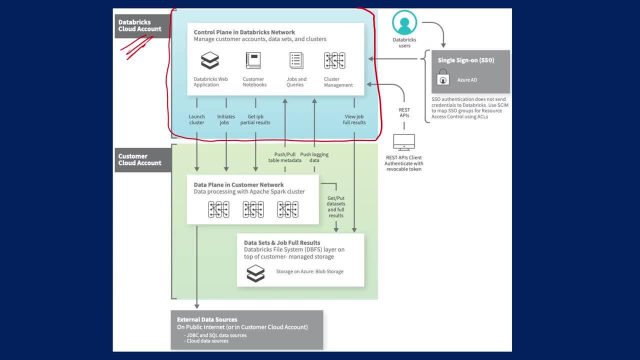 Cloud, That means Azure Databricks as a service. it itself will contain one cloud account, So there it will keep all the control plane, which will contain all the backend things- what you need for your Databricks account to work properly. 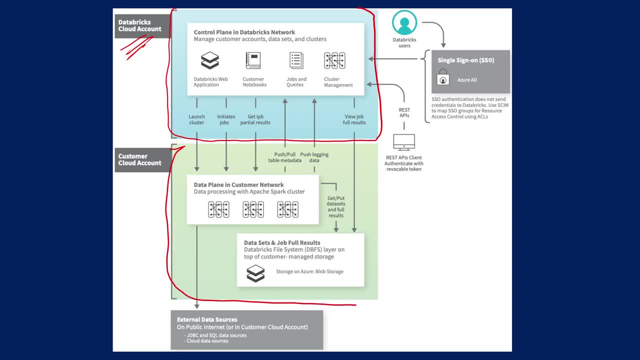 And you will have something called data plane, and the data plane will be in the customer's own Azure account. Okay, So now what will happen in the control pane? So whenever we open Databricks, it will open in a browser with a UI and everything right. 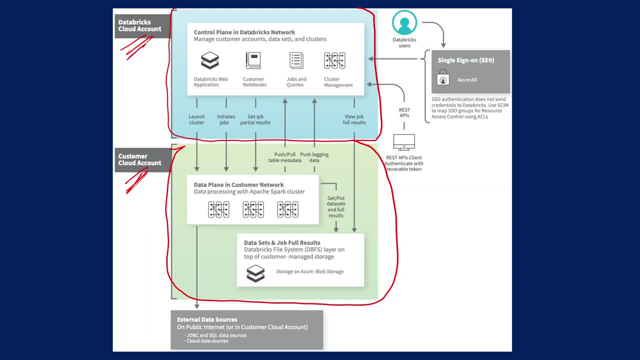 All that the Databricks UI is. it is nothing but like a web application, only right So that The application related information will be in the control pane. Not only that, the customer created notebooks also will be in the control pane. 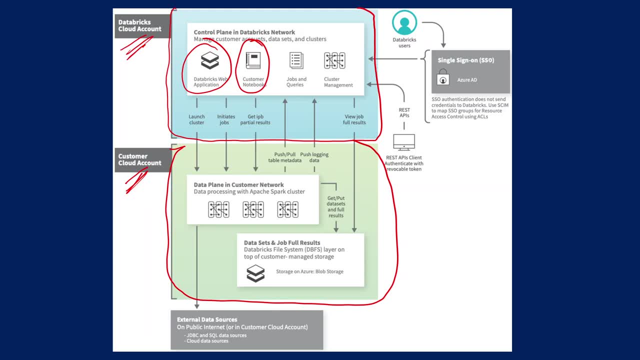 Not only that: in the workspace, once you create a notebook, you will schedule the jobs and everything right. So all that information will be available in the control pane only. It will be stored in the control pane in an encrypted fashion. And also control pane contains something called cluster management. 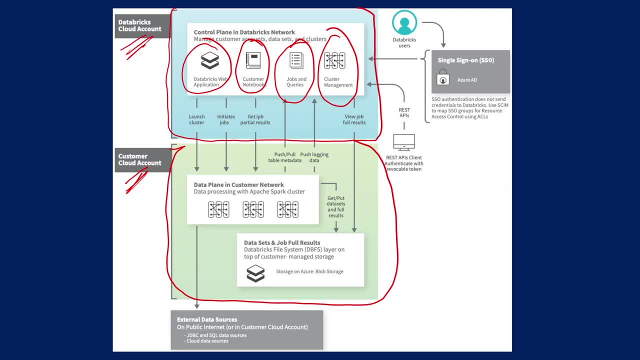 So this cluster management is the one that will make sure the clusters to run and everything right. So by the word it is making clear: right, It is a cluster management, It is a cluster management system. okay, And in the data plane, as I said, data plane is within the customer network. 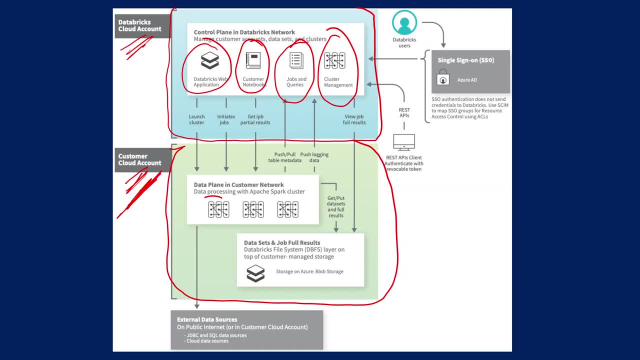 That means it is within your customer's cloud account And here clusters will be there and these clusters will take the data and perform the data processing. okay, So data processing will actually happen in the data pane. So this is like a data pane. 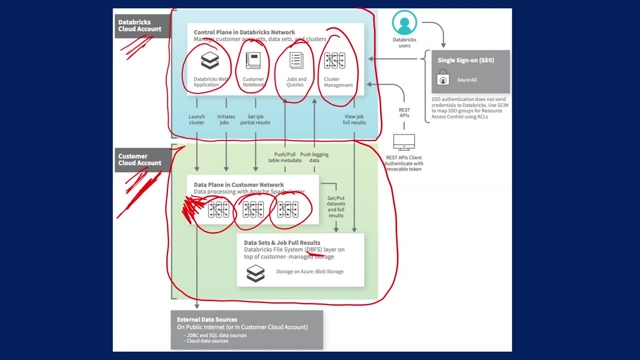 And also in the data pane. only you will have something called Databricks file system. In our past videos in our past videos- the last video, the seventh video- what we did, We kind of uploaded one file into DBFS, right. 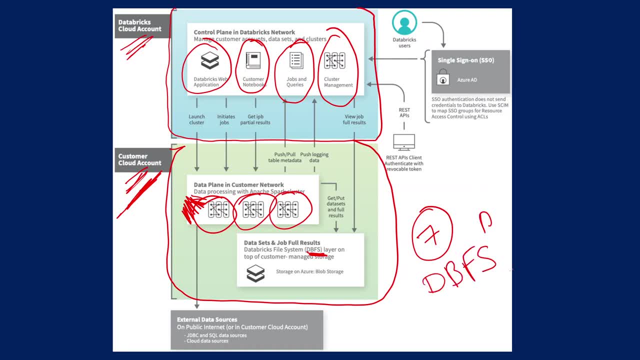 Databricks file system right. So from that storage we tried to read the data right. So DBFS is a thing like for now. think like it's like your Databricks account. whatever you create that account's own storage, personal storage. you can think like that. 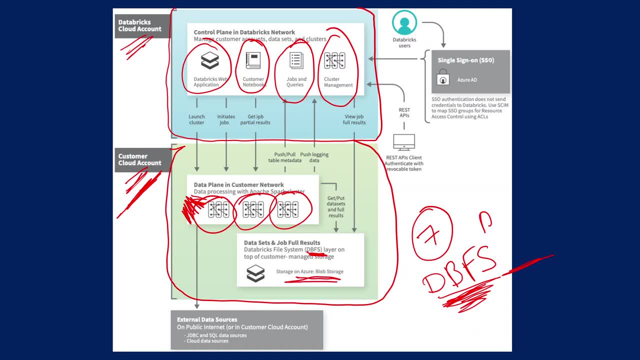 In the backend. what will happen? actually, that is actually a Azure blob storage. only Within your own Azure account it will create one Azure blob storage And top of that blob storage it will create a layer that will be called as Databricks file system. 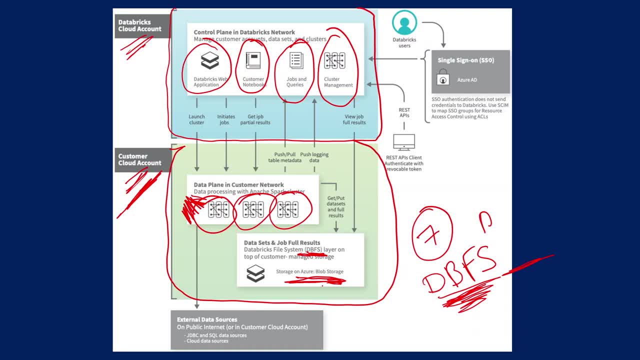 We will discuss about this Databricks file system in detail. For now, think like Databricks file system will be Databricks account's own storage layer where you can upload the data and then take the data for your data processing and all. 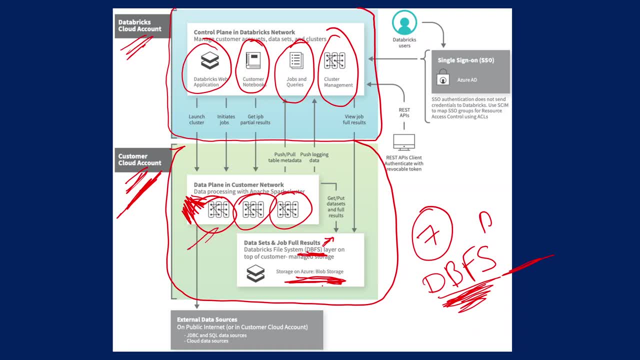 So this is Databricks file system and this data processing logic and where your data resides. everything will be in the data pane only And the rest everything, all the backend services, So what Databricks account needed to work, and all the customer notes, books and the job related information and the login related information. everything will be stored in the control pane. 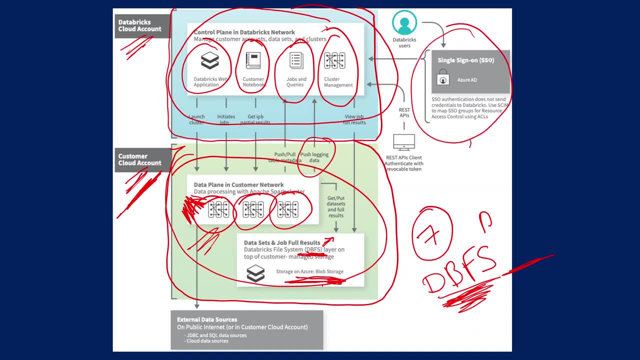 So and yeah, so this is like a single sign on using which any customer can connect to Azure Databricks. So this is what the high level architecture of the Azure Databricks account. uh, no need to go very deep into it for now. 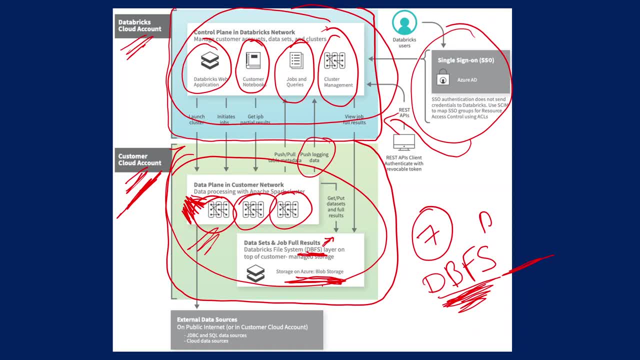 I mean, if you get a clear idea, like okay, there is something called two things, One is control pane, another one is data plane control pane, the one where all the databricks- web application code and also the customers notebook, whatever we develop, and also the jobs related information, logging related information, cluster management. 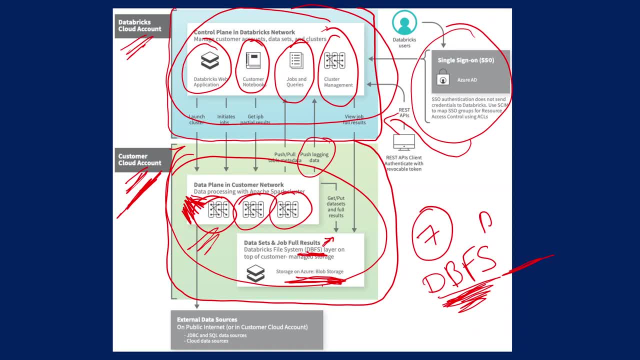 so everything will be there in the control pane and this control plane will be in the azure's own cloud account. and now second thing is customers own cloud account. so here the data plane will be there in in the data plane. only customers data will be managed completely. data will not move. 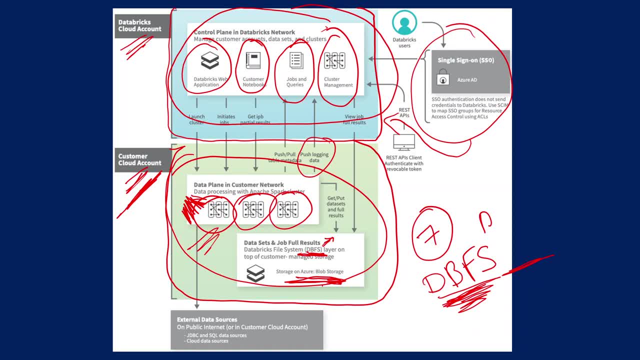 to control plane. so your customer data processing and storing and connecting the external resources and fetching the data and storing data to the external resources. everything will happen through data plane. only so to do that, databricks have something called connectors. actually, so to connect to the external sources, databricks use the some connectors, using that connectors. 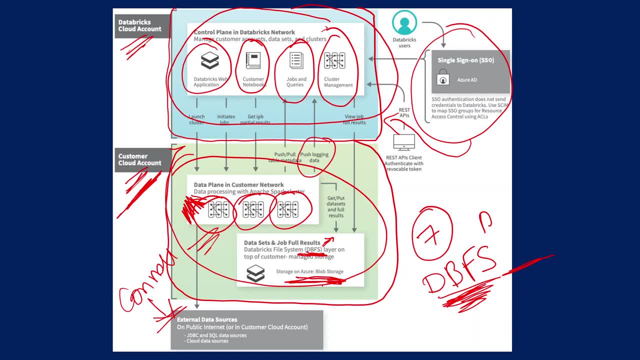 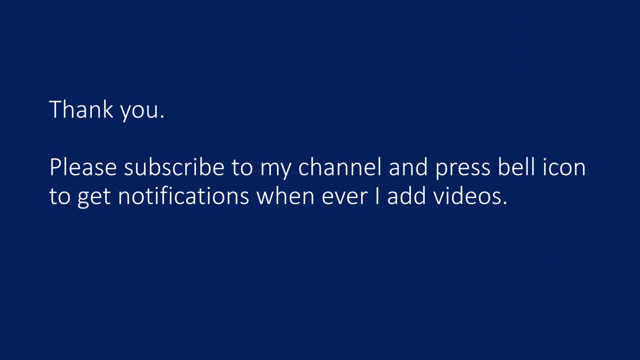 you can connect to the external resources and get the data or load the data to you, so we will discuss everything in detail in our upcoming videos. i hope you got a basic idea about the database architecture and a high level. thank you for watching this video. please subscribe to my. 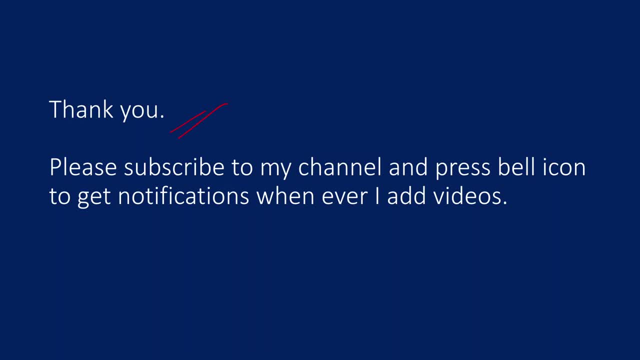 channel and press the bell icon to get the notification whenever i do this. thank you so much.